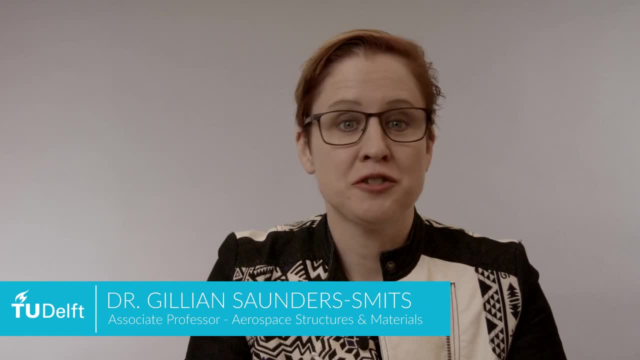 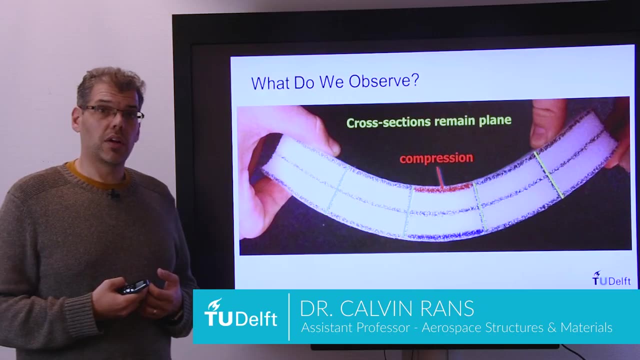 Hi, my name is Gillian Sonner-Schmidt and I am a professor in Aerospace Structures and Materials here at Delft University of Technology. Together with my fellow professors from the Department of Aerospace Structures and Materials of the Faculty of Aerospace Engineering at Delft University of Technology, we will take 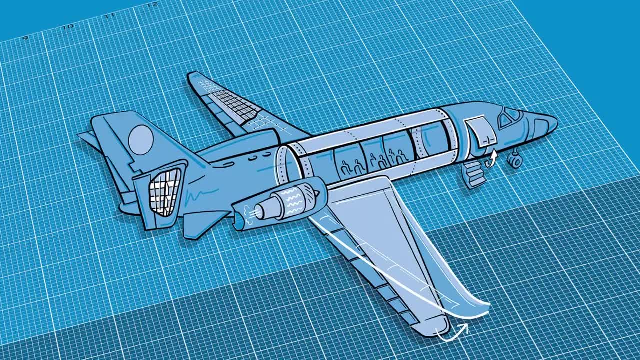 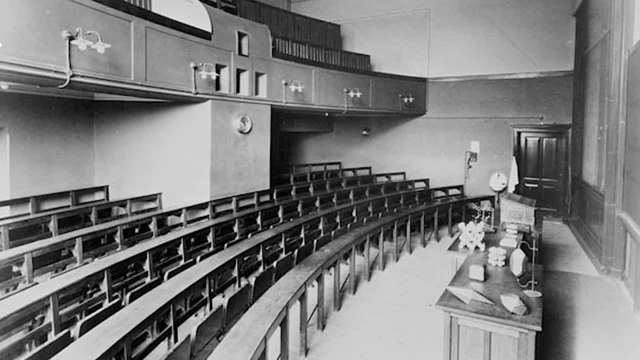 you on a journey through the considerations behind the structural and mechanical design of aerospace vehicles in our course Introduction to Aerospace Structures and Materials. This course is one of the oldest courses taught here in Delft, having been part of our curriculum since 1945. 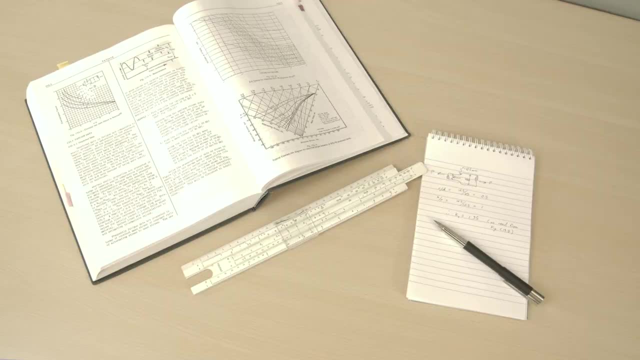 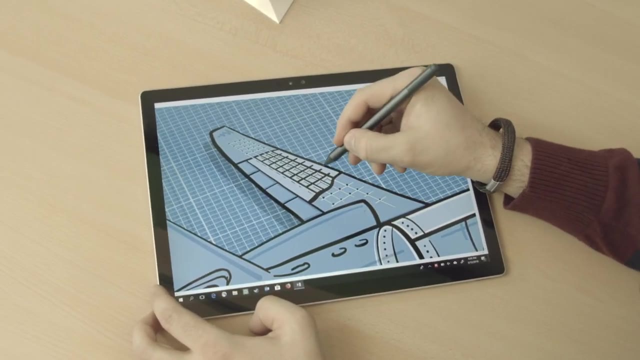 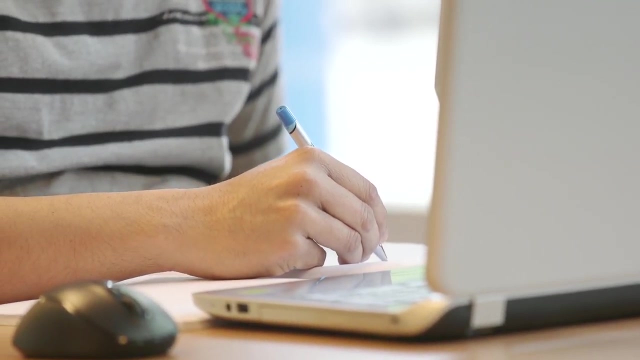 This doesn't mean, however, that the course is only for beginners. The course is old-fashioned. Instead, like aerospace, the course has evolved through the years. It enables students to understand and explain the principles of aerospace, structural and materials design. Now we are taking this course on its next incarnation by going online, allowing the 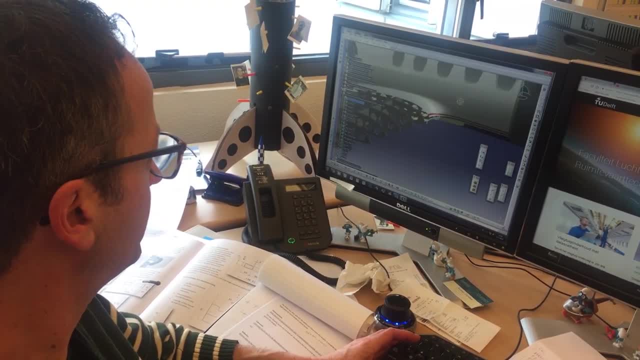 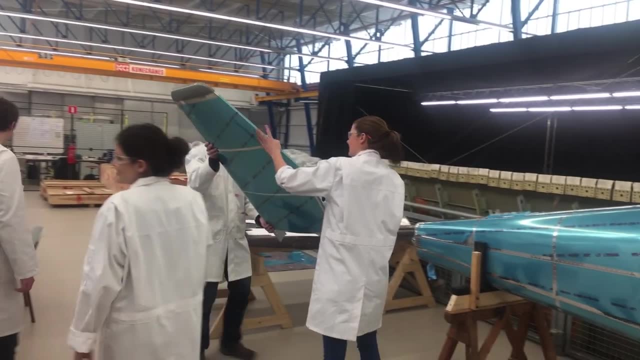 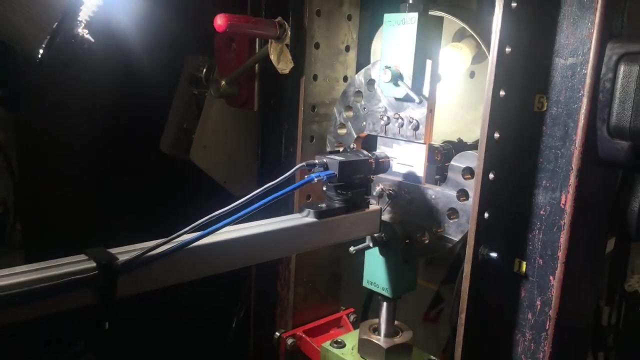 whole world to learn, think, analyze and design like an aerospace structural and materials engineer. During the course, you will learn to analyze structural design problems, philosophize about material choices and make manufacturing decisions, Taking into account the latest developments in the aerospace field and giving you access. 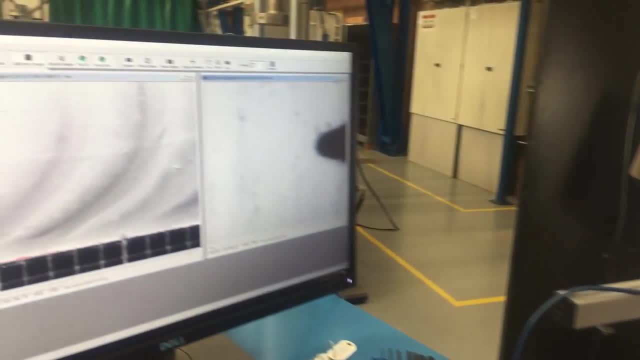 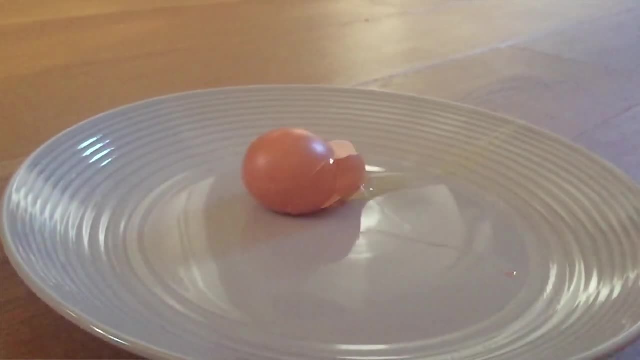 to the most recent research by our Structures and Materials experts right here at TU Delft. We will not just explain theory, but also show you experiments, some of which you will be able to repeat at home by yourself, so that you can really get a feel for the matter. 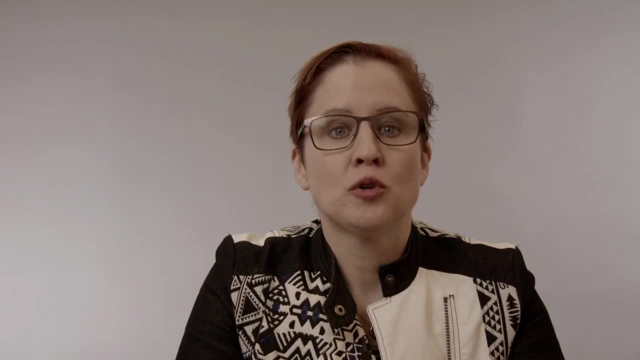 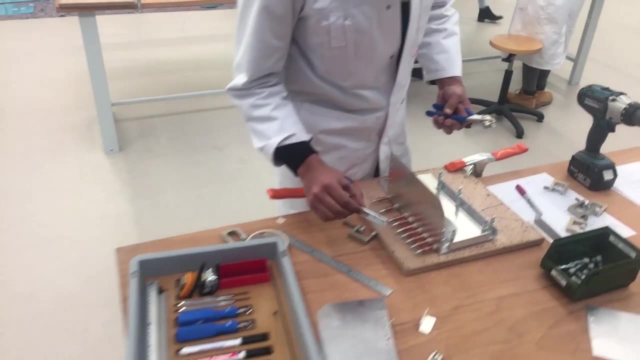 at hand. Next to that, we will confront you with the dilemmas we aerospace structures and materials engineers face when making design choices balancing not only weight and costs, but also issues like availability, structural and material limitations and manufactory abilities, whilst 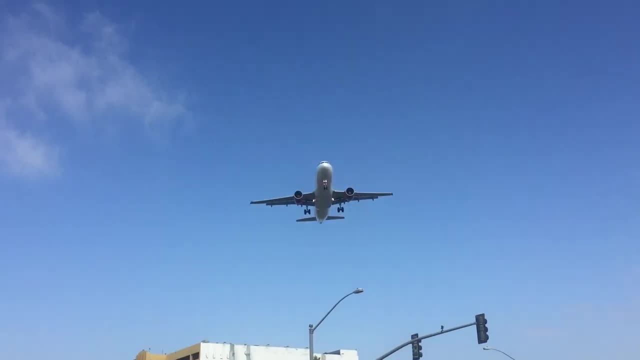 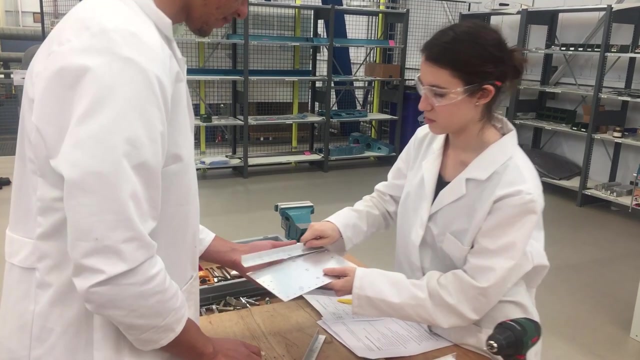 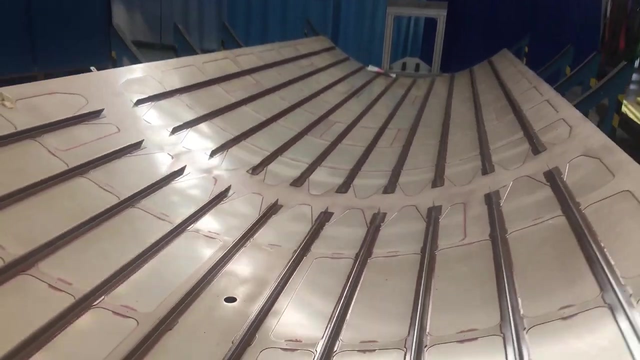 ensuring the safety and durability of aircraft and spacecraft in their ever-varying operating environment. In this course, you will think of design solutions to aerospace structural and material problems, challenge your creativity and test your innovation and problem-solving skills to come up with solutions for the multi-faceted issues at hand. 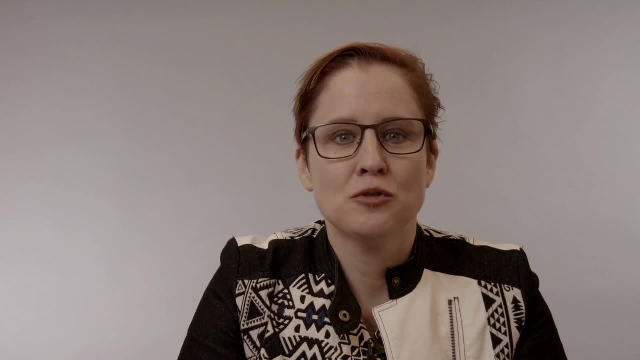 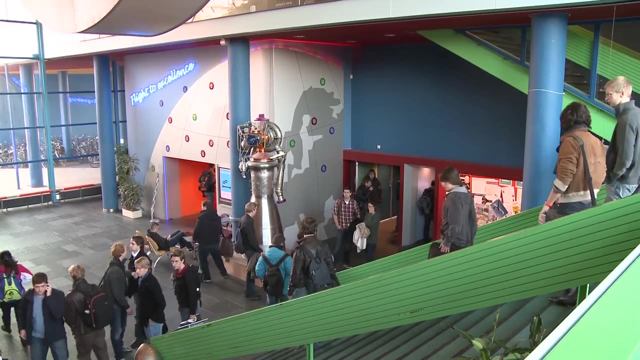 Have you got what it takes to join us in coming up with the best solution for the design of safe aerospace vehicles? Then join us and share in our passion for aerospace structures and materials by taking this course. We look forward to seeing you on board our course soon.